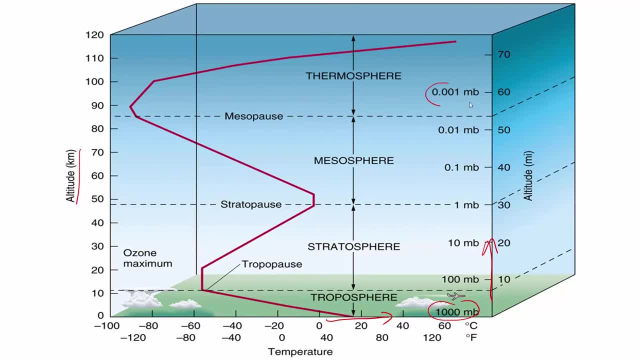 you go above, as you can see, the temperature drops off down to almost zero as you get into something called the thermosphere. So where do we start? Near the surface, we have a layer called the troposphere, which is where all the weather and climate happens, as we can see from these clouds. This is where 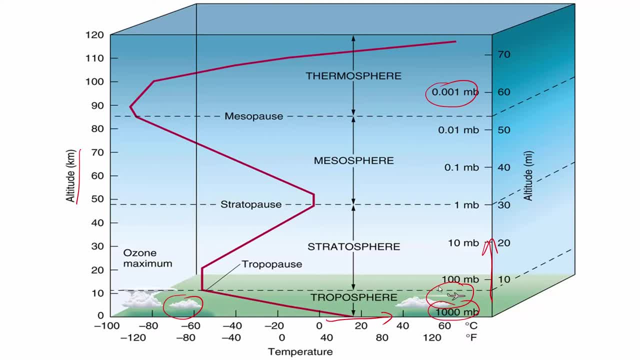 most of the airplanes fly as we see the picture here, And above the troposphere there is a dividing line called the tropopause, Above which you have another layer called the stratosphere, And above the stratosphere again you have a stratopause, a mesosphere, mesopause, and 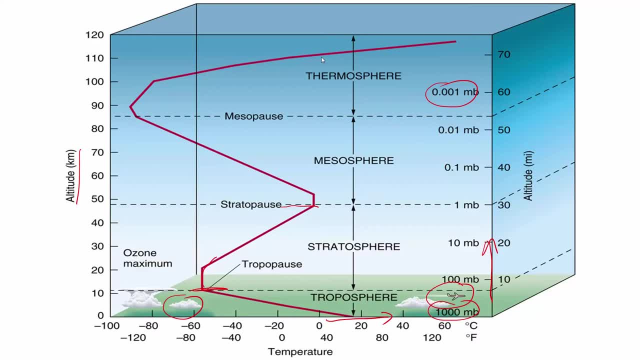 a thermosphere. The density of the air also begins to drop as we go above The fewer and fewer molecules in the upper atmosphere. So if we start from the troposphere, all the radiation from the sun that is coming in, all the way from gamma rays and X-rays- 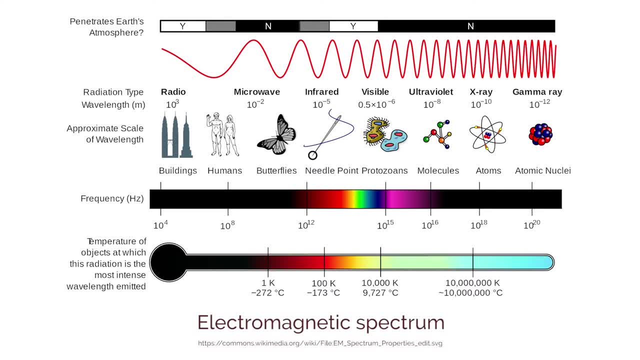 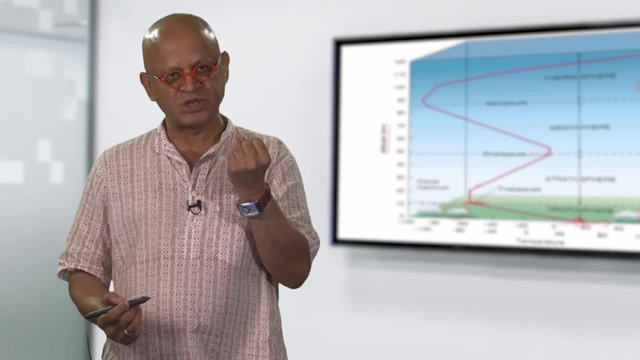 To UV radiation, to visible radiation, to long wave radiation or infrared radiation, and then microwaves and radio waves and so on. Most of the visible radiation is reaching all the way to the surface, basically because the atmosphere is not absorbing much of it. 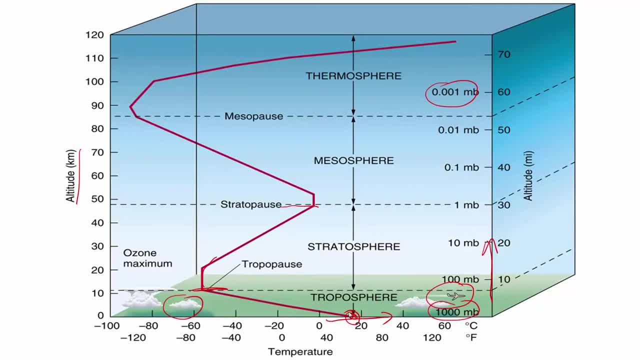 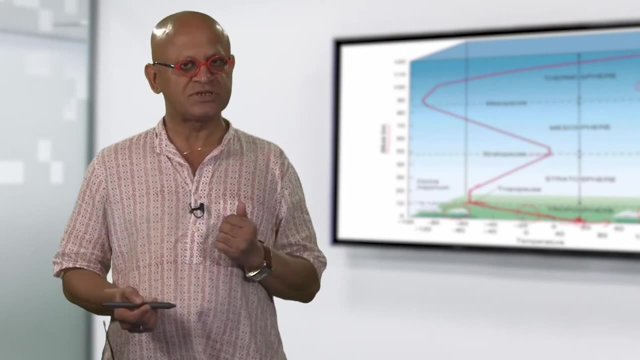 That energy is warming the surface. so you can see that the troposphere is, on average, about 18 degrees centigrade near the surface. As we go from the surface towards the tropopause, the temperature drops because it gets colder, So the pressure is dropping and the temperature. 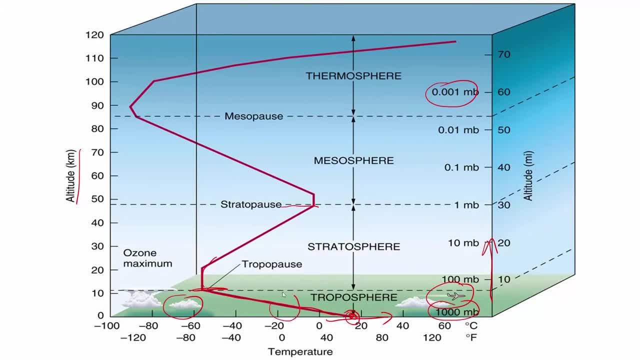 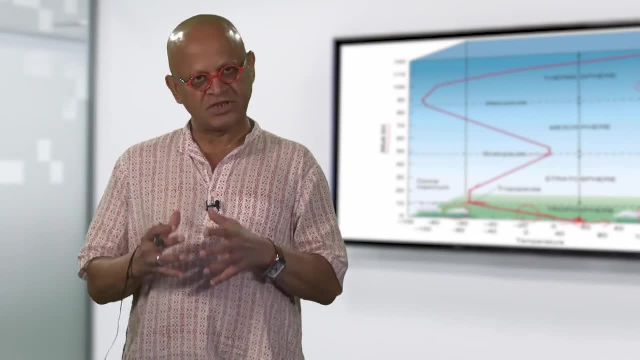 is dropping. This is where most of the humidity in the system lives And we will see in other modules that the humidity is higher in the tropics because the temperatures are warmer. It will get drier and colder at the poles. So wherever you have, 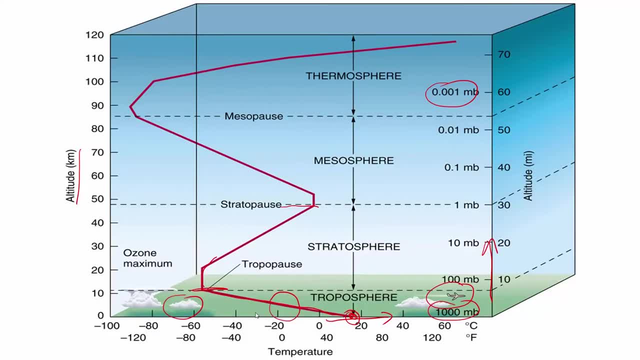 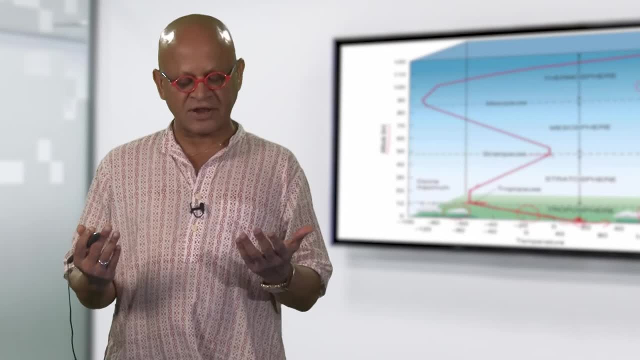 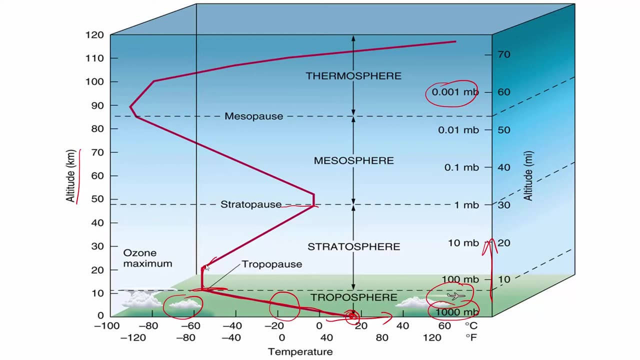 humidity in the atmosphere, you are going to have condensation, hence clouds and rain In the stratosphere. it is called stratosphere because the Greek word stratos means stratified, So it is got a different temperature gradient: It is colder at the bottom and warmer at the top. Basically because the UV energy from the sun can interact with the oxygen molecules in the stratosphere, split it into oxygen atoms which can combine with another oxygen molecule and form ozone. And ozone is almost opaque to UV, Which means it will absorb almost all of the UV radiation, Which is a good thing because 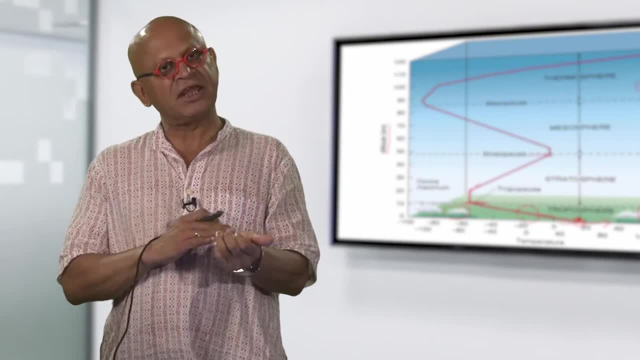 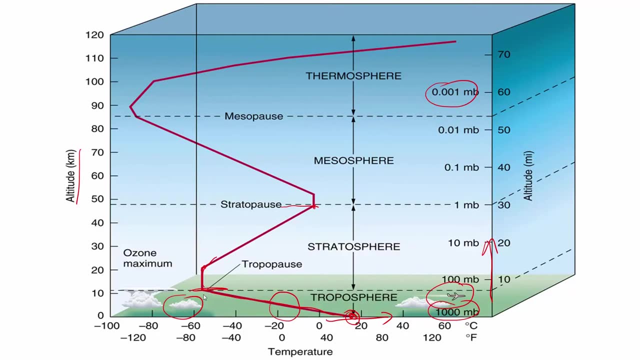 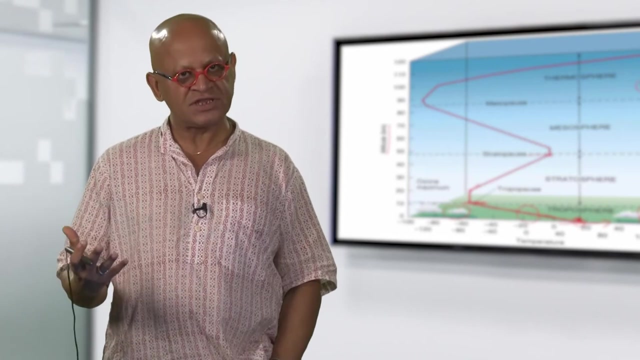 if UV comes into the lower atmosphere, then it can actually burn our skin and we can get cancer and so on. So the troposphere is basically consisting of everything we can think of, Not just human habitation, but all the forests. Most of the mountains are obviously within the tropopause. 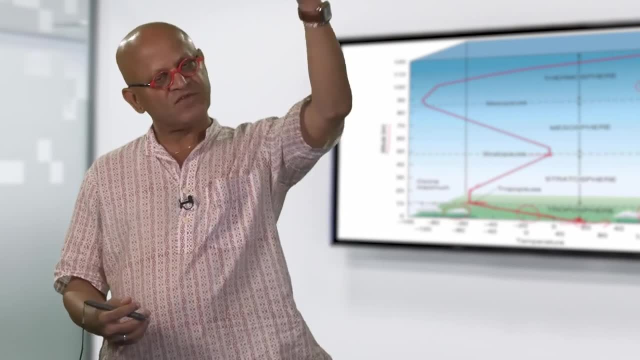 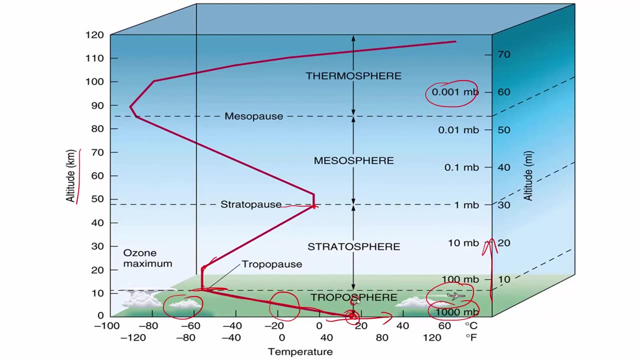 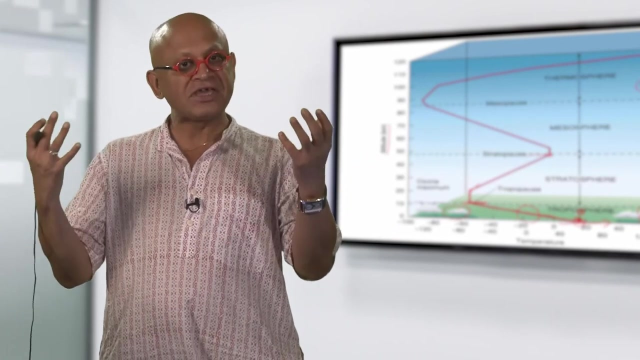 And when volcanoes go off, for example, Most of the volcanoes go above the troposphere into the stratosphere. So anything that is thrown into the troposphere can get rained out or can get deposited, Whereas if you put something in the stratosphere it can stay for a long time. So if a volcano puts dust, 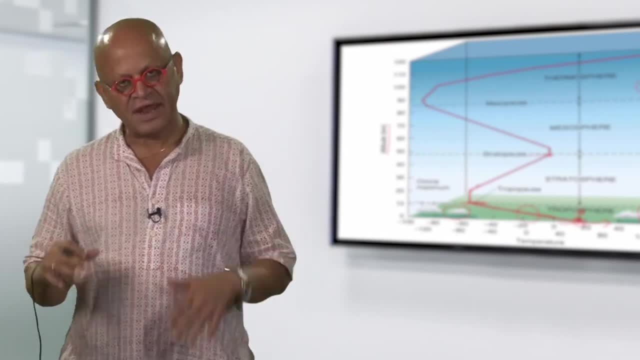 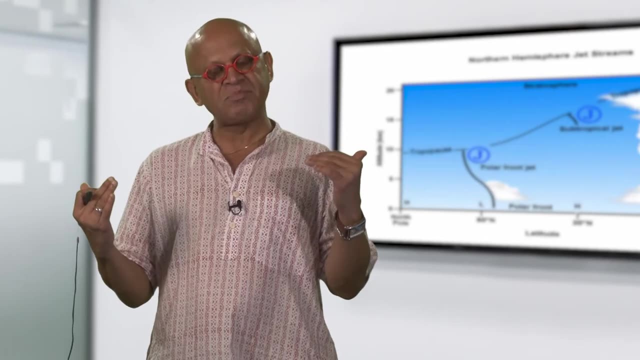 into the stratosphere. it can stay there for a long time and can cool the atmosphere, as we will see in another module. So what happens to this tropopause and the temperature gradient? We have a sort of gradient as we go from the equator towards the pole. We know that the 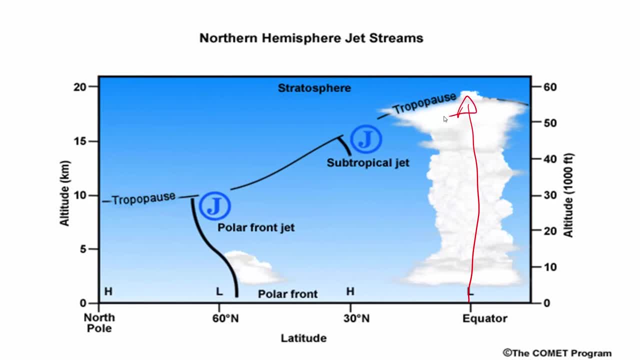 equator is warm, So the tropopause is high because the warm air is expanding and it is occupying more volume. But as you go to higher latitudes the temperature gets colder, So the tropopause also gets colder. So by the time you reach the poles the tropopause is 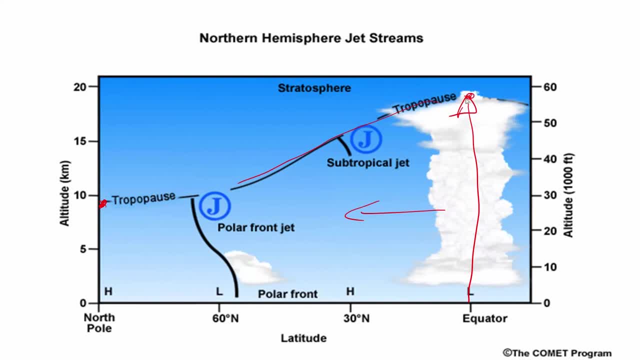 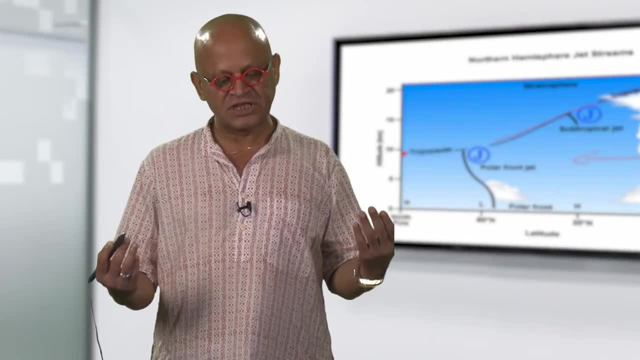 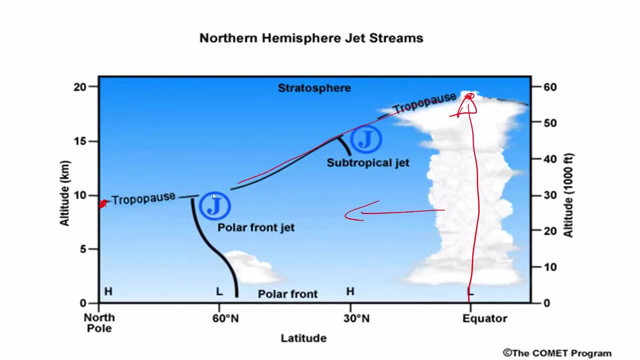 about 8 to 9 kilometers, whereas near the equator, in the tropics, the tropopause is almost 8- 12 kilometers high. this can have consequences that we will see in other modules, in terms of where it rains, how much it rains, etc. and you have to think about what happens to this.